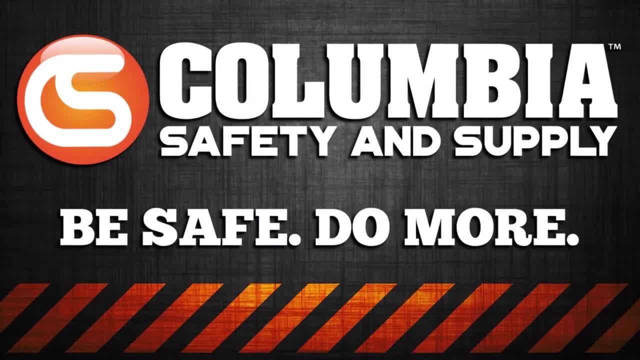 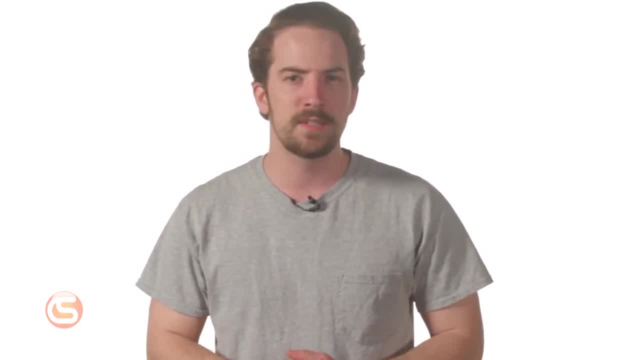 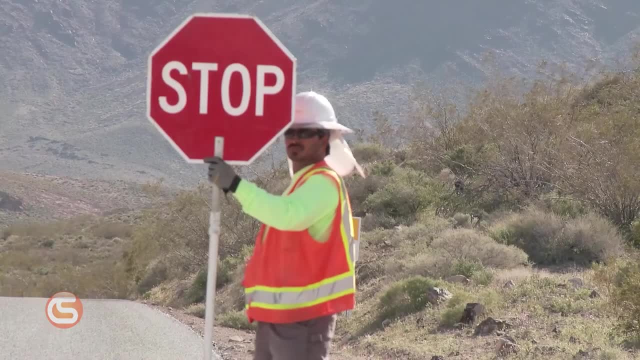 I'm Connor with Columbia Safety and Supply, and today we're going to talk about the Manual on Uniform Traffic Control Devices, or, as it's better known, the MUTCD. The MUTCD is the written regulation on traffic signs, lights and other traffic control devices. It is a national standard. 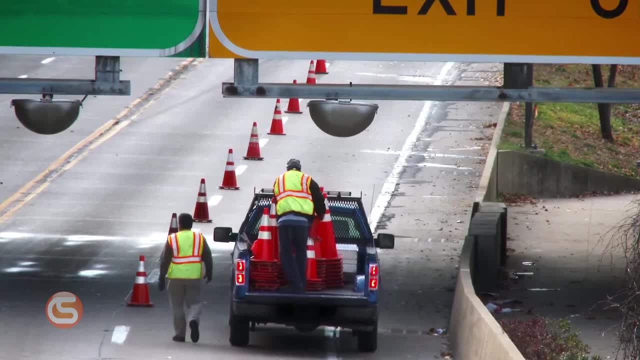 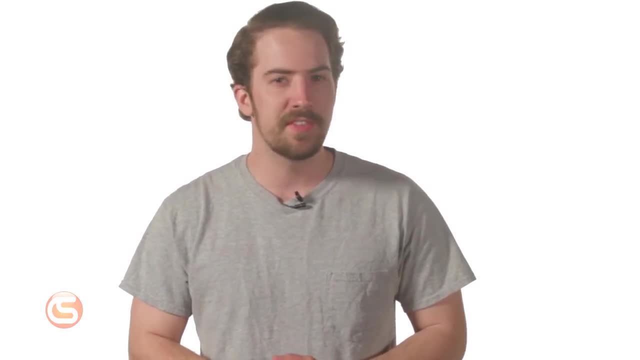 however, most states supplement it with their own standards to meet specific needs. While the average person may think that the size, color and shape of traffic control devices are simply to maximize visibility, most of them have a much more specific meaning In this video. 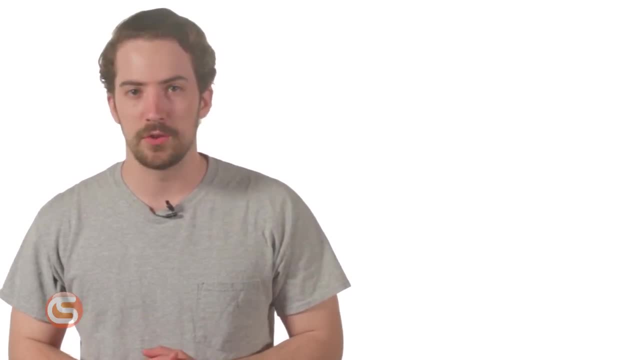 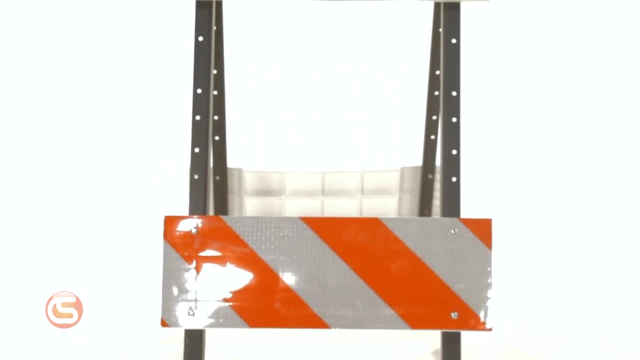 we're going to explain the MUTCD standard for some of the more common traffic control devices. First, let's take a look at barricades. Barricades are designed to communicate road closings, restricted areas and delineate changes in road lanes. They must be self-standing. 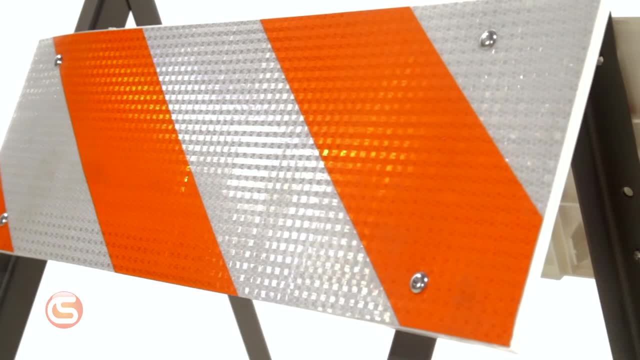 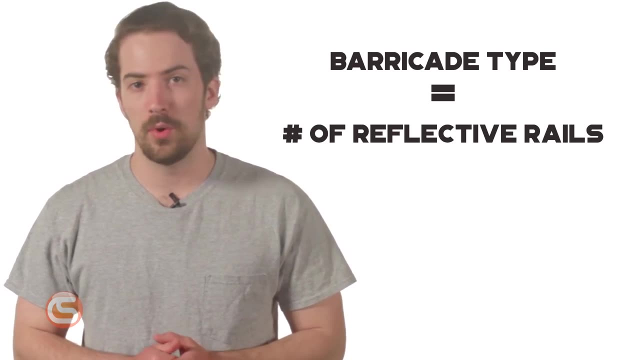 have a minimum rail length of 24 inches and include at least one rail with alternating orange and white retroreflective tape. The number of reflective rails on a barricade determines which type it is. one, two or three Type 1 are used for conventional. 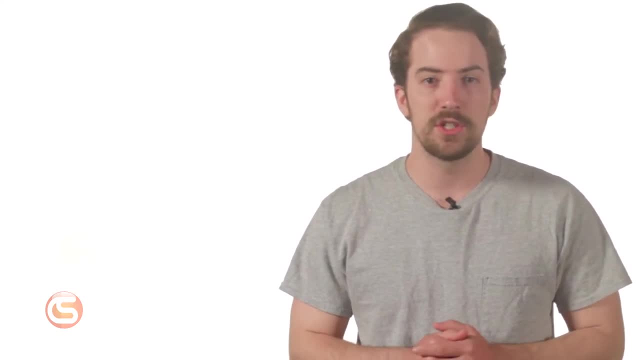 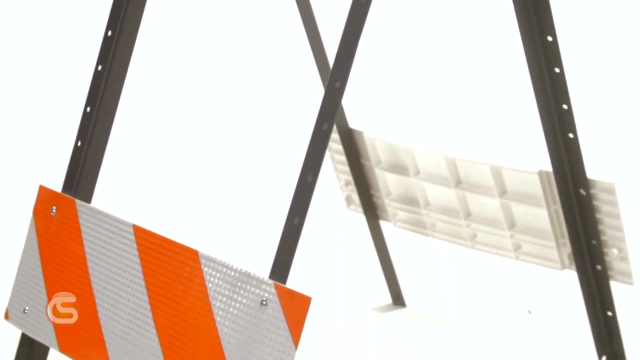 roads and urban streets. They require one 8 to 12 inch reflective rail face on each side. Type 2 is intended for freeways and higher speed roadways where traffic is maintained through the work zone. These must have two retroreflective rails on each side. Type 3 barricades are specifically. 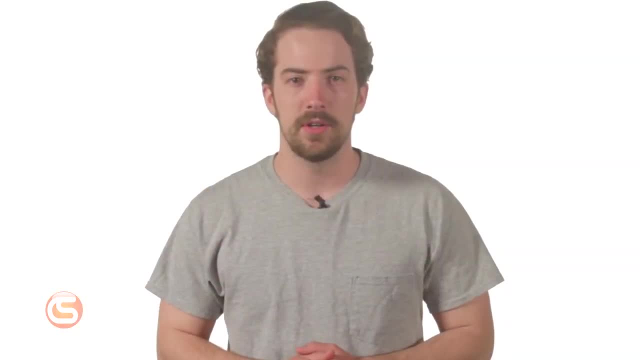 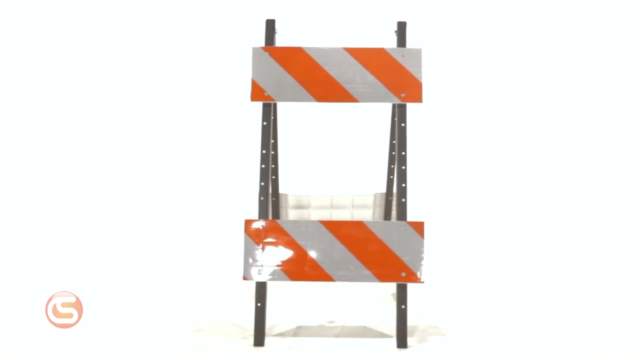 used for complete road closures and may extend across the entire road. These barriers must have three reflective panels on each side. If you pay close attention, the stripes on the panels will be pointing in a specific direction. This indicates the intended path around them in Type 1 and Type 2. 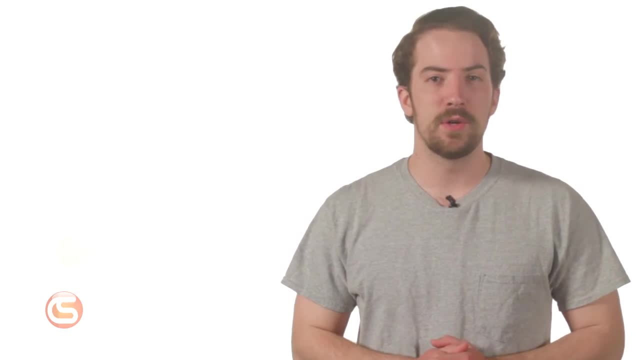 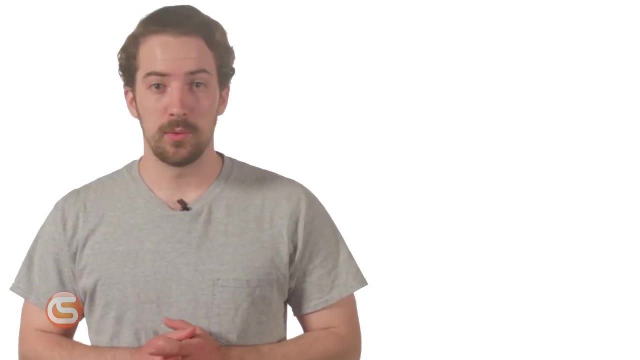 versions. Next we'll take a look at traffic cones. The purpose of traffic cones is to channelize traffic, divide traffic lanes and delineate short-term maintenance or utility work. But not any old sports cone will work for this. They must be at least 18 inches tall and 28 inches tall on. 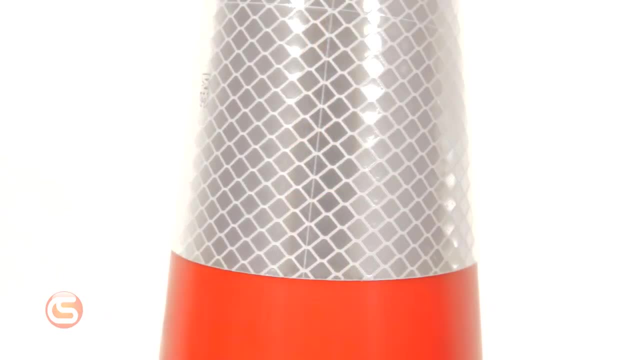 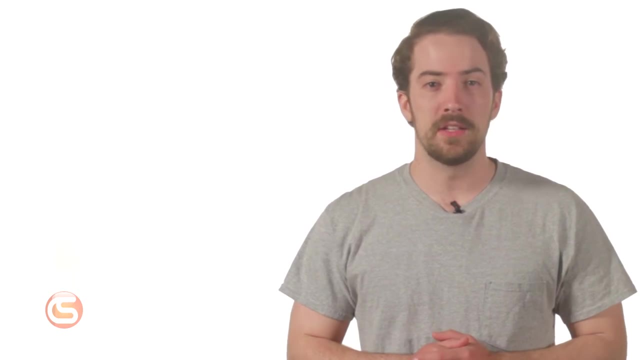 roadways where speeds exceed 45 miles an hour. They must also be crash-worthy. Essentially, they'll either collapse or bounce away if struck by a car, causing minimal damage to the vehicle. The design of them must be predominantly orange and have some kind of weighted base or measure. 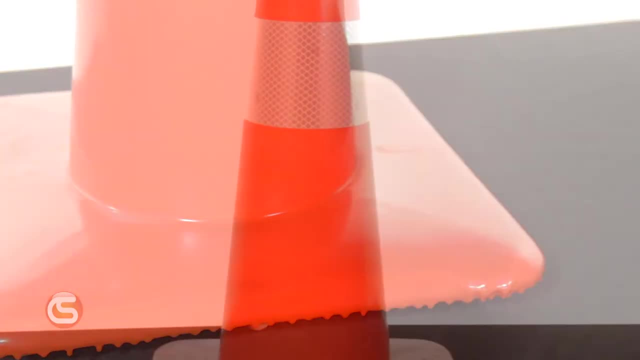 to keep them standing At night. cones must be equipped with a high-pressure, low-pressure or low-pressure system or be equipped with lighting devices or retroreflective bands. On those 28-inch cones, the retroreflective band must be 6 inches wide, no more than 4 inches from.